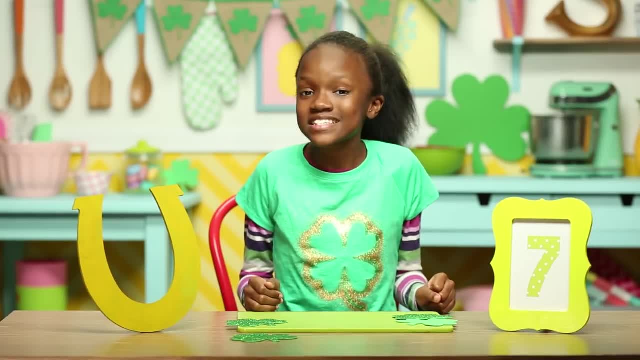 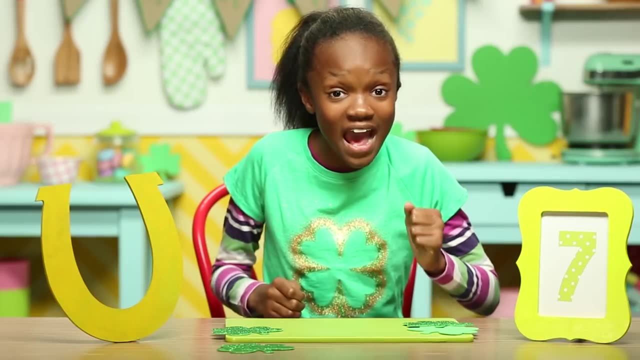 Hackey St Patrick's Day, or, as I call it, St Hat-trick's Day. I'm on a lookout for a leprechaun, so they can lead me to a pot of gold. Legend has it: the more charms you wear, the better chance you have at finding one. 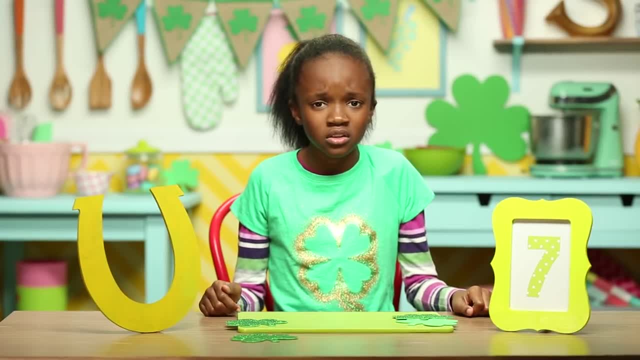 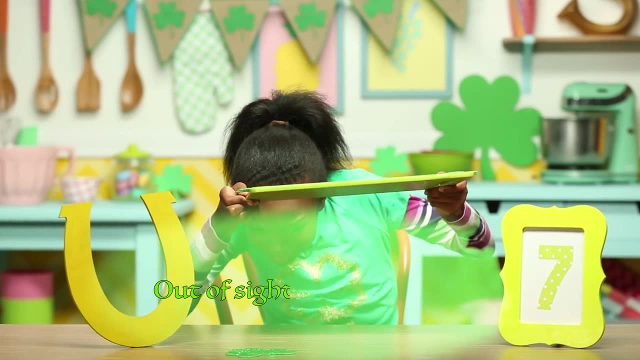 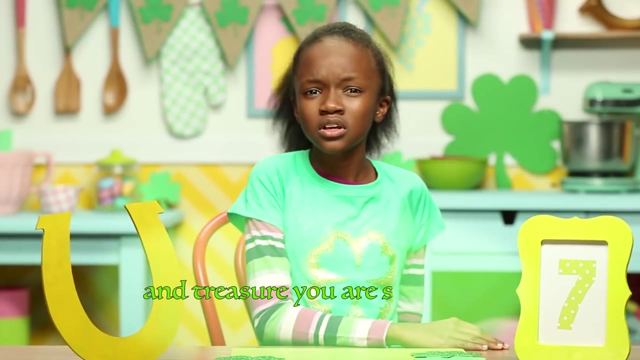 But so far I hadn't had any luck. Did somebody say a leprechaun, What? Where Out of sight, not out of mind, a pot of gold you wish to find? Hack these clues and riddles three and treasures, you are sure to see. 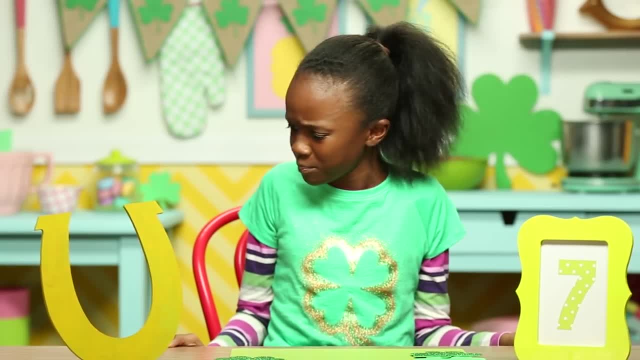 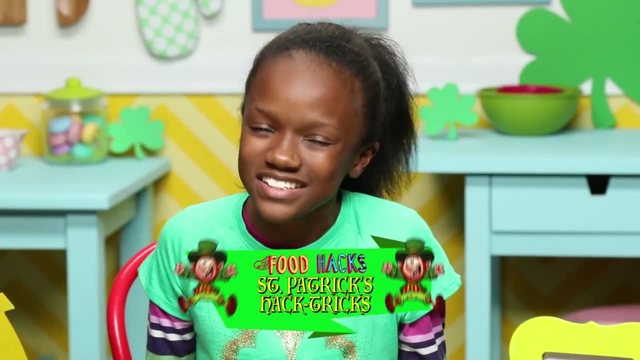 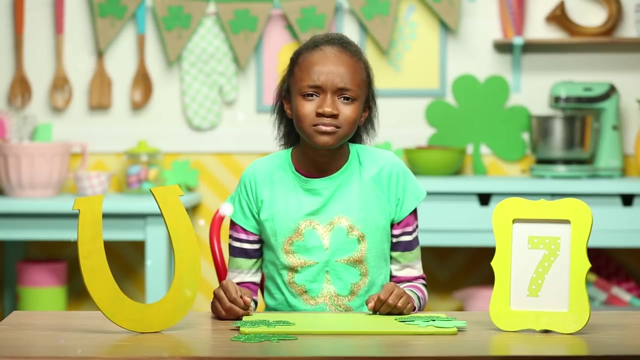 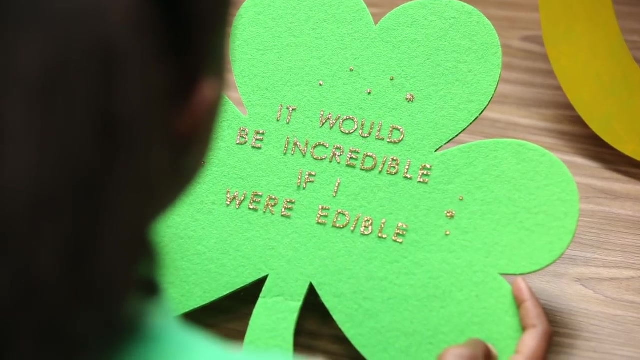 So you give me clues and I have to food hack them Easy. I do this every day. Looks like today's episode is St Patrick's Hack-tricks. So where's my first clue? Oh, it would be incredible if I were edible. 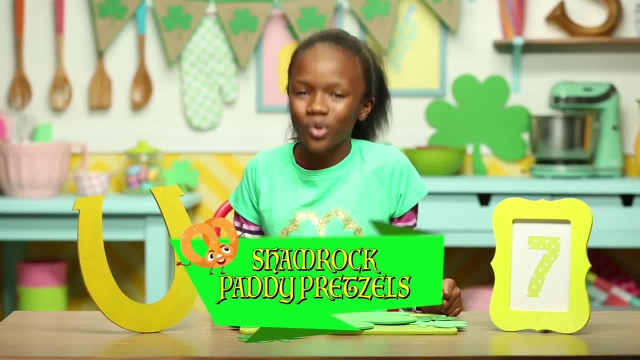 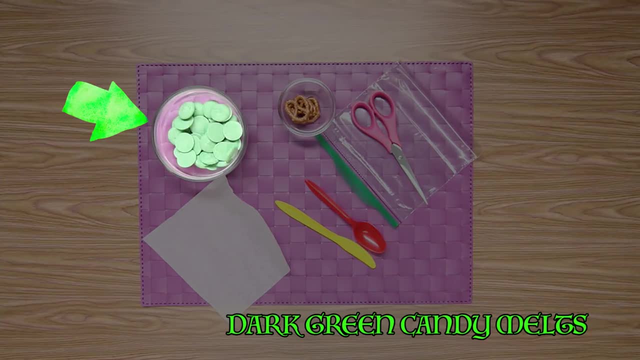 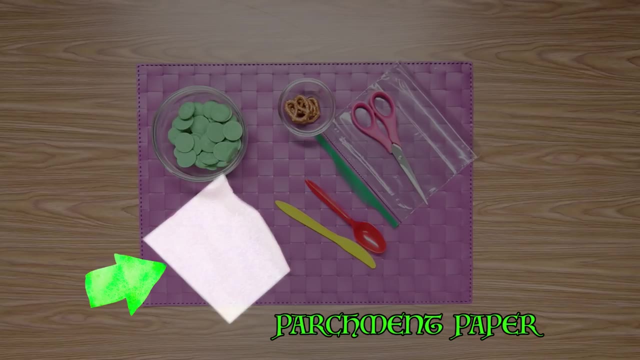 Looks like we're hacking some shamrock patty pretzels. For this you'll need four small pretzel twists, dark green candy melts, a Ziploc bag, scissors, a knife, a spoon and parchment paper. Lay three pretzels in the shape. 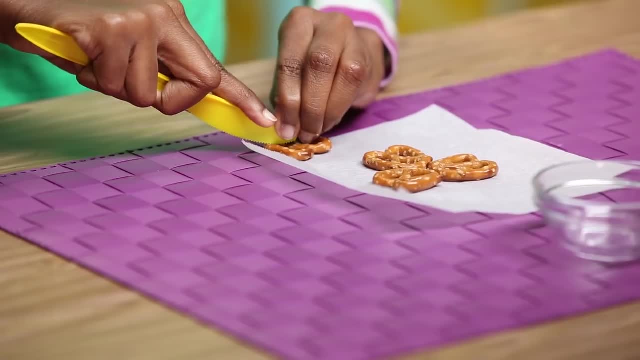 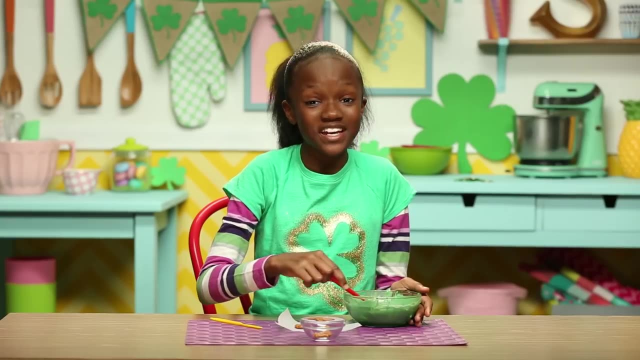 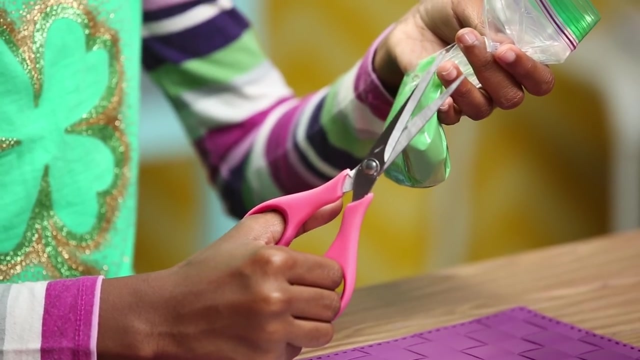 of a shamrock on your parchment paper. Cut a piece off of your other pretzel like this, for the stem. Melt your candy melts in the microwave. Put your melted candy melts in your Ziploc bag and cut off the tip. Squeeze your candy melts onto the pretzels, like this: 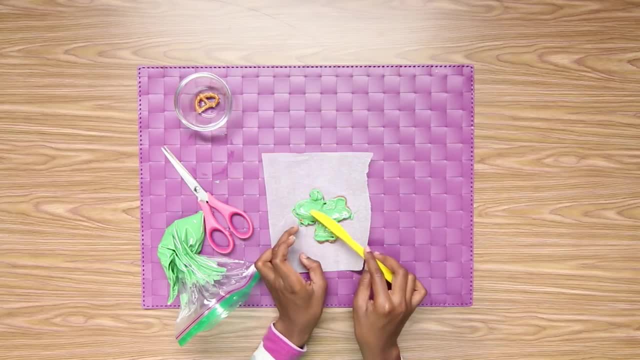 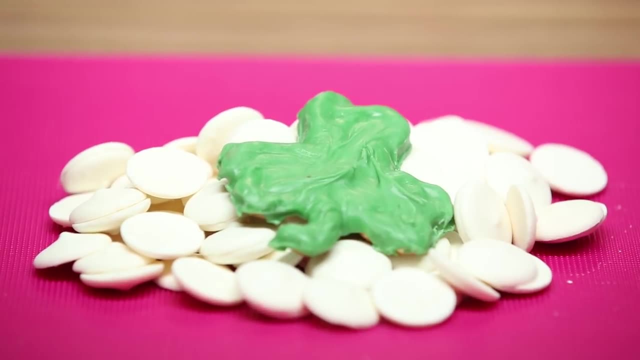 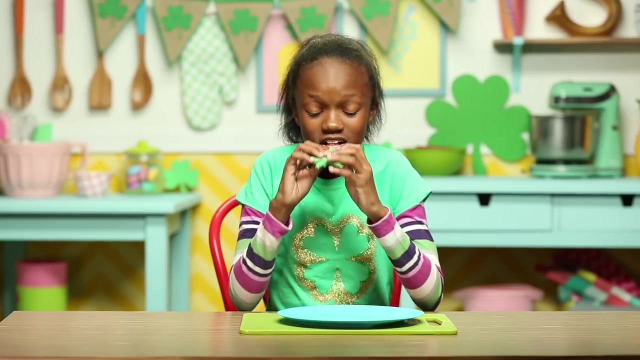 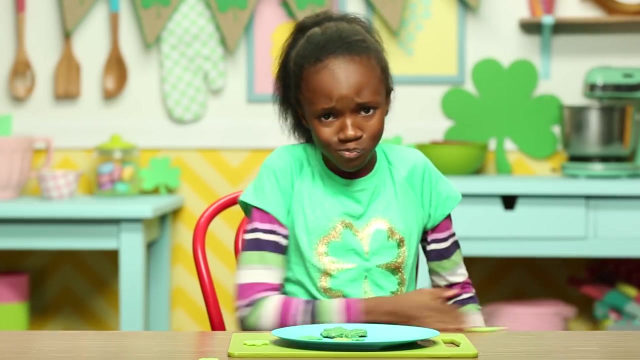 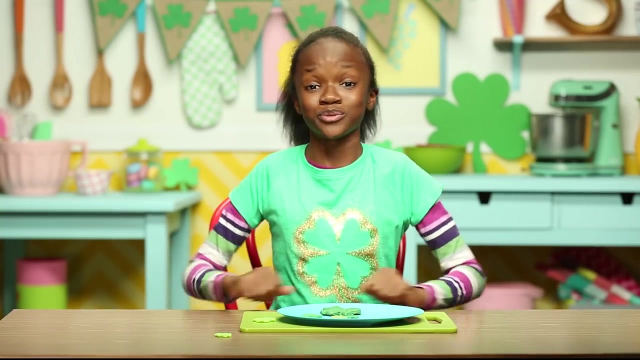 Use a knife to help you spread it around evenly. Now let it harden. Well, I have to try one to make sure they are good enough. zh aha, I heard leprechauns were tricksters. Okay, so she obviously wants me to hack a hat. 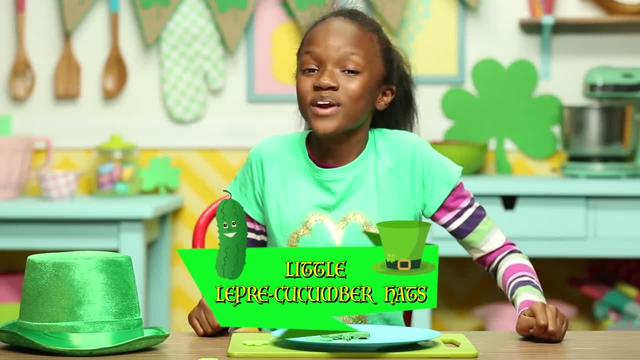 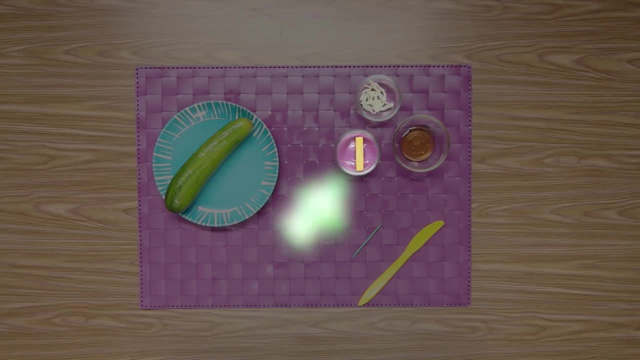 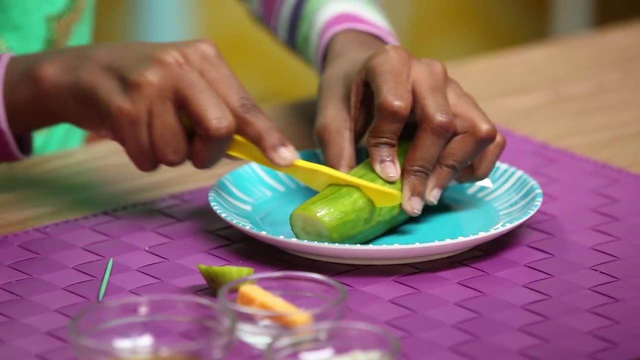 No problemo, One little leopard cucumber hat coming up. For this you'll need some cucumber, cheddar cheese, shredded mozzarella, a little bit of honey, a knife and a toothpick. Cut a piece of cucumber about one inch tall like this: 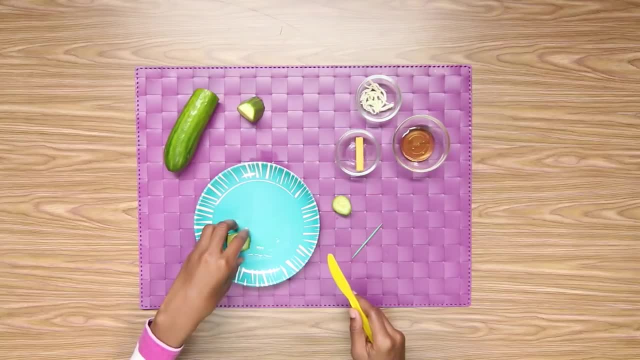 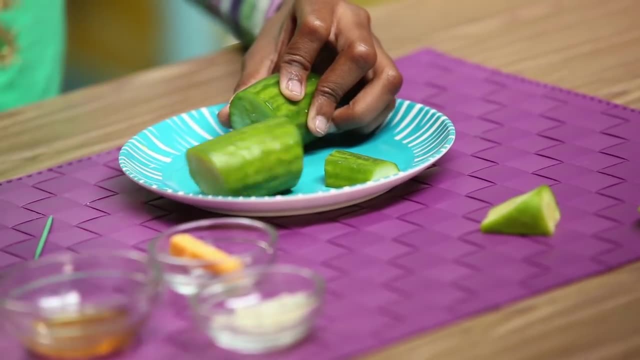 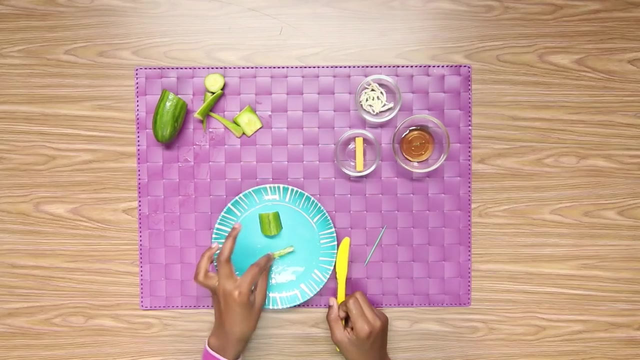 Then cut that piece in half. Lay one piece flat-side down. Now cut a piece of cucumber that's slightly larger than your first piece. Cut that piece in half, then cut a skinny strip. This will be the brim of the hat. 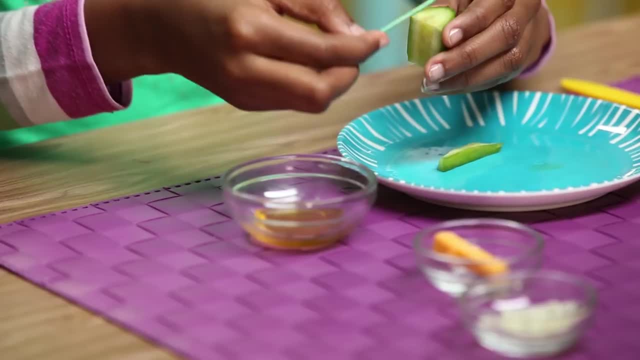 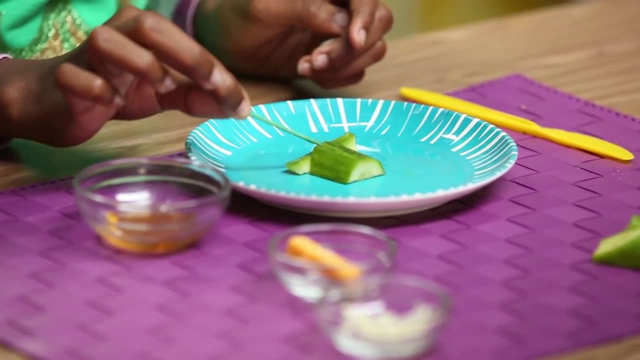 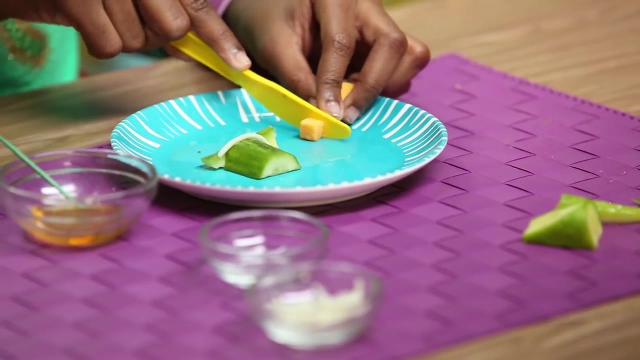 Use your toothpick and some honey to put the cucumber pieces together. Now spread some honey along the seam of the hat And lay a piece of shredded cheese on top. Cut a small square of cheddar cheese. Use honey to stick it onto the seam like this. 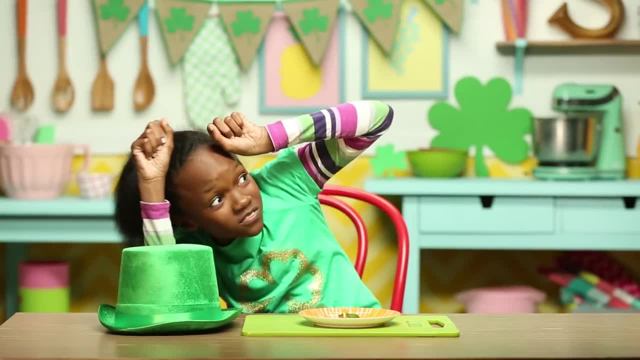 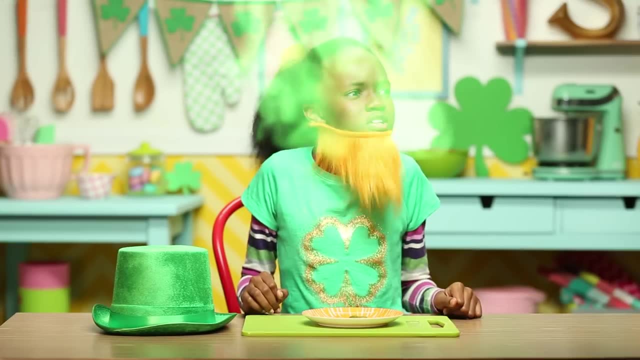 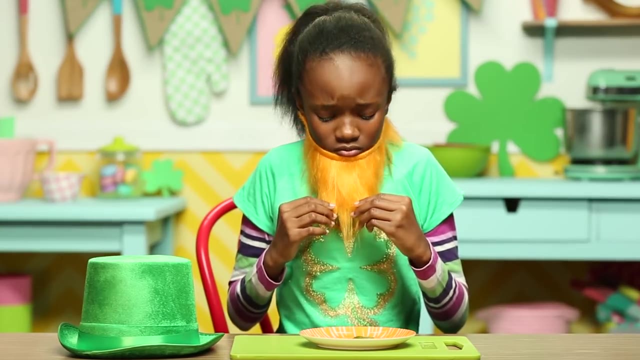 Delicious. Whew, I thought for sure she would trick me again. Hee, hee, hee, hee, hee hee. What? I heard that? What A beard. Let's get back to hacking. There's a pot of gold calling my name. 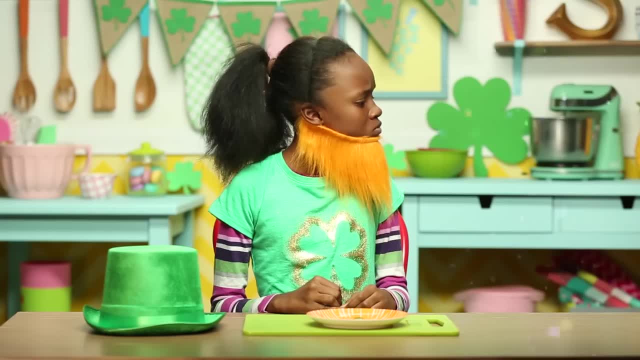 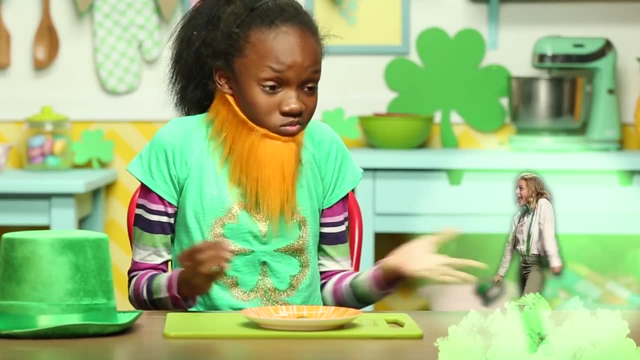 Shannon, Shannon, Wait, you're the leprechaun. Yeah, I'm a leprechaun. My name's Ally, by the way. Oh, OK, Ally, What's left? Well? Well, I've got one more thing to do. 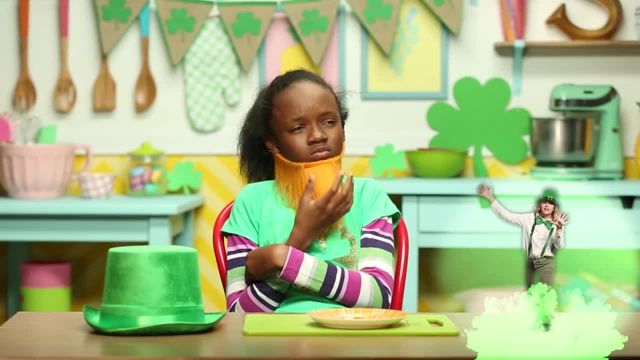 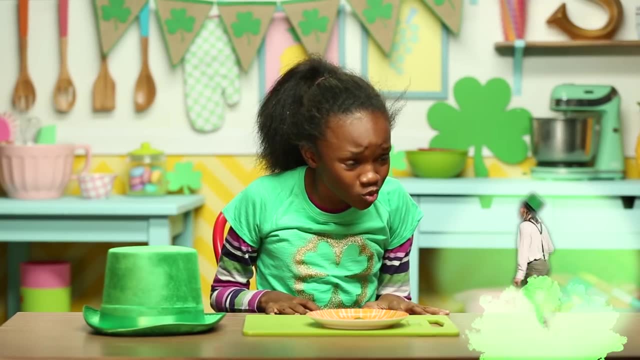 Well, I've got one more thing to do: clue a riddle to solve what lies at the end of a multicolored fog. is it a pot of gold? it's a pot of gold, right? hmm, I don't know. wait, yes, you do, just make the. 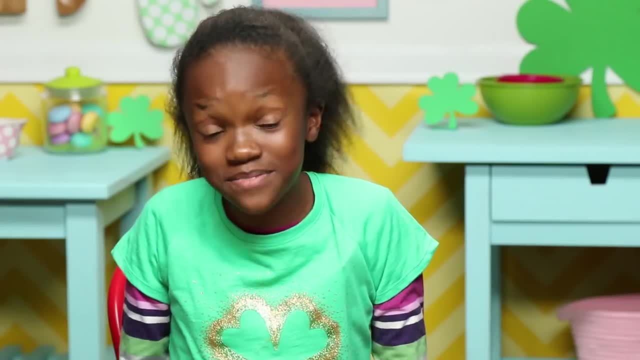 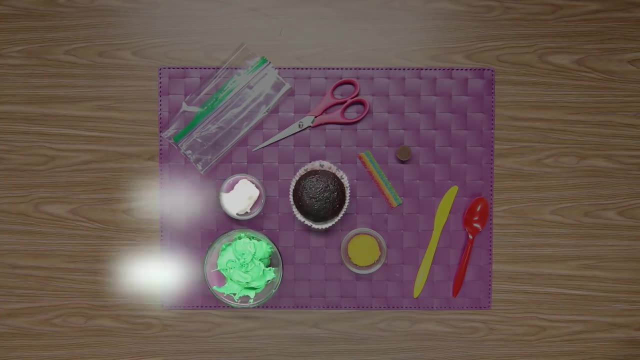 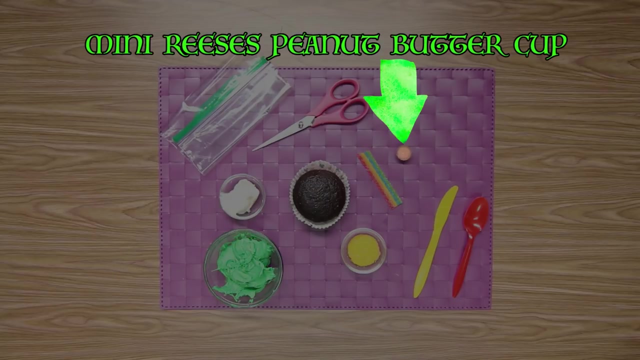 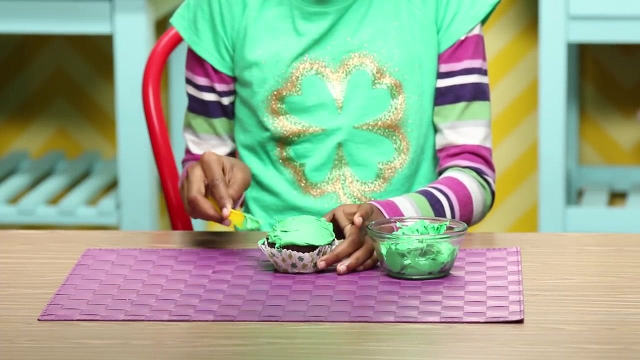 hack. let's make my pot of gold pastries. for this you'll need a chocolate cupcake, green and white frosting, a rainbow candy belt, a Reese's miniature peanut butter cup, yellow sugar sprinkles, a ziploc bag, some scissors, a knife and a spoon. frost your cupcake with the green icing, then set it aside. take your peanut.